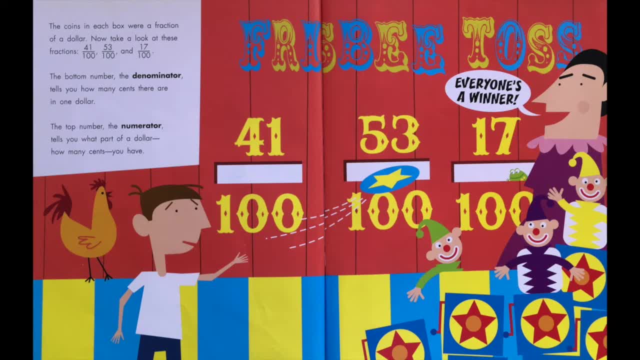 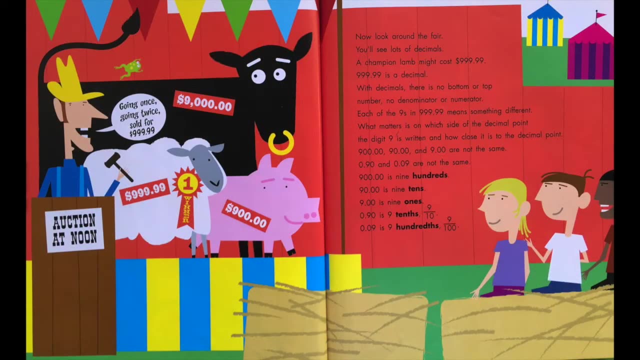 The bottom number, the denominator, tells you how many cents there are in one dollar. The top number, the numerator, tells you what part of a dollar there is, How many cents you have. Now look around the fair. You'll see lots of decimals. 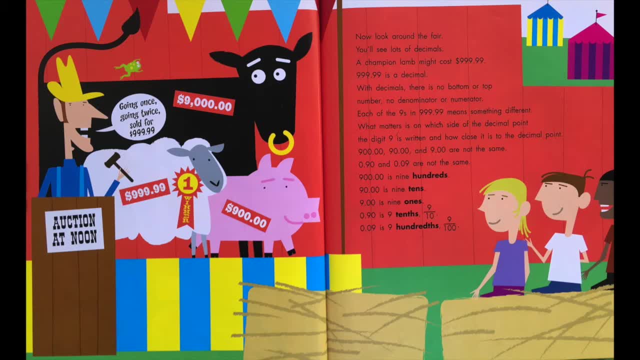 A champion lamb might cost $999.99.. $999.99 is a decimal. With decimal there is no bottom or top number, no denominator or numerator. Each of the nines in $999.99 means something different. $999.99 is differenceable. 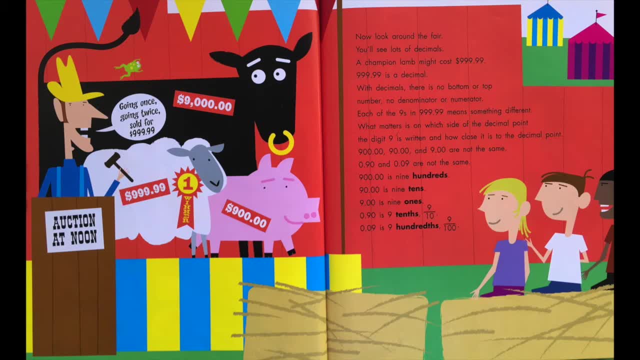 What matters is on which side of the decimal point the digit 9 is written and how close it is to the decimal point. 900.00,, 90.00, and 9.00 are not the same. 0.90 and 0.09 are not the same. 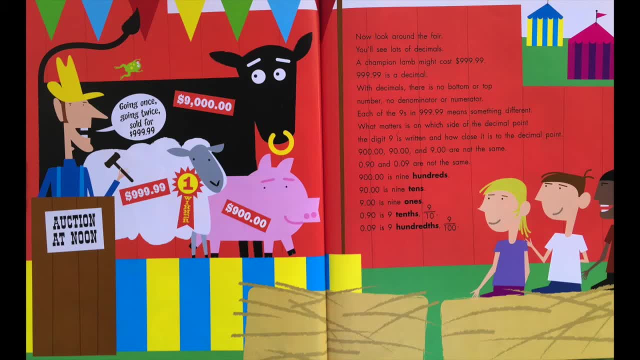 900.00 is 9 hundredths, 90.00 is 9 tenths, 9.00 is 9 ones, 0.90 is 9 tenths or 9 over 10, and 0.09 is 9 hundredths 9 over a hundredth. 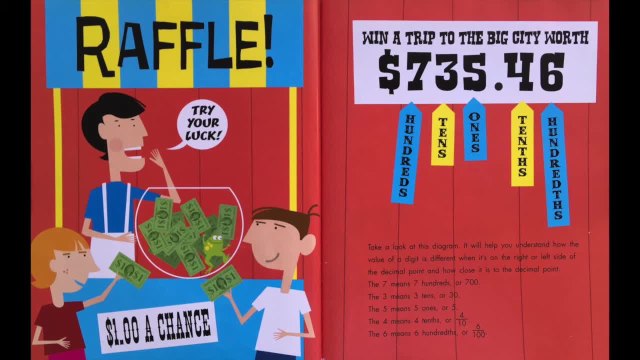 Take a look at this diagram. It will help you understand how the value of a digit is different when it's on the right or left side of the decimal point and how close it is to the decimal point. The 7 means 7 hundredths or 700,. the 3 means 3 tens or 30,. the 5 means 5 ones or 5 dollars. 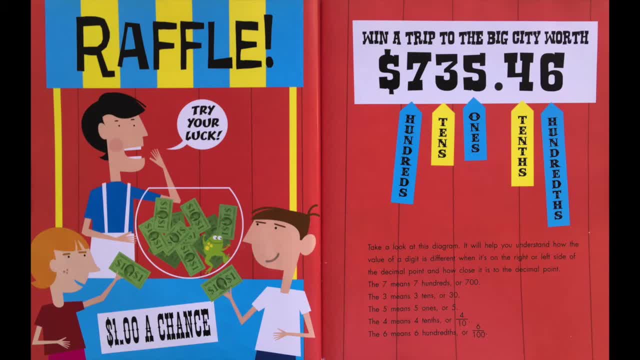 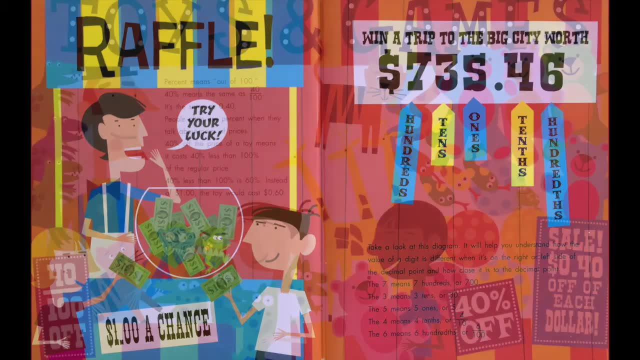 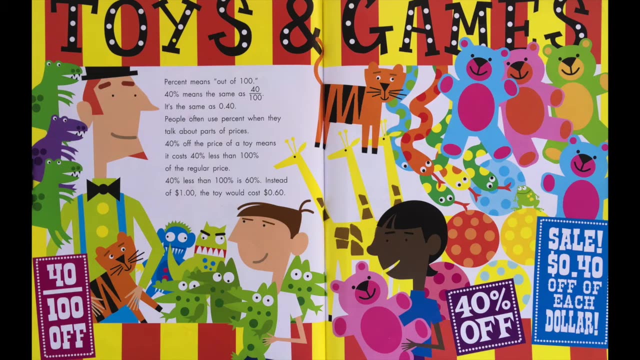 the 4 means 4 tenths, or 4 over 10, and the 6 means 6 hundredths or 6 over a hundredth. Percent means out of a hundred. Forty percent means the same as 100.. It's the same as 0.40.. 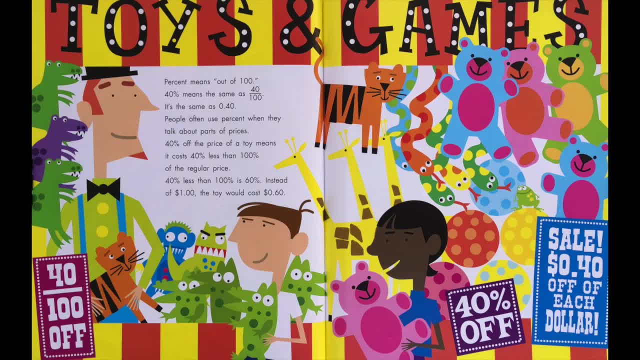 People often use percent when they talk about parts of prices. Forty percent off the price of a toy means it costs 40 percent less than 100 percent of the regular price. Forty percent less than 100 percent is 60 percent. Instead of a dollar, the toy would cost 60 cents. 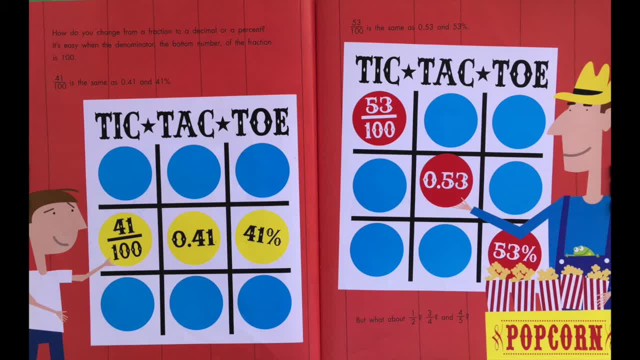 How do you change from a fraction to a decimal or a percent? It's easy with a denominator. The bottom number of the fraction is 100.. 41 over 100 is the same as 0.41 and 41 percent. 53 over 100 is the same as 0.53 and 53 percent. 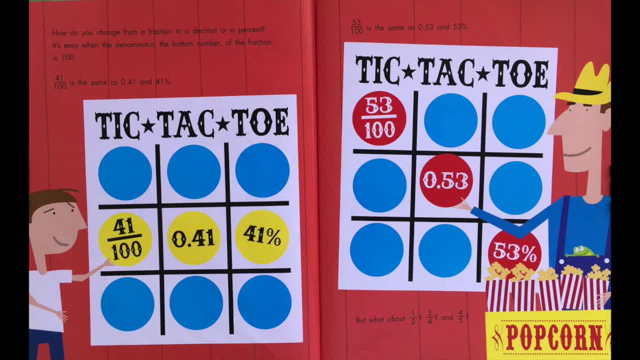 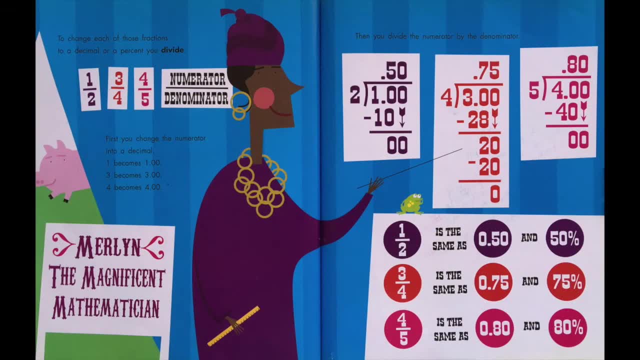 But what about 1 half or 3 fourths and 4 fifths? To change each of those fractions to a decimal or a percent, you divide First. you change the numerator into a decimal: 1 becomes 1.00,, 3 becomes 3.00, and 4 becomes 4.00.. 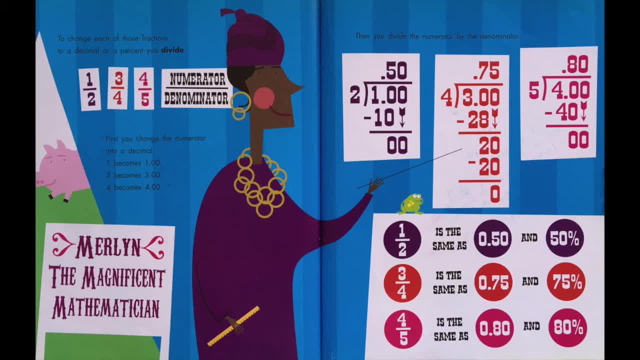 Then you divide the numerator by the denominator. One half is the same as 0.50 and 50 percent. 3 fourths is the same as 0.75 and 75 percent. 4 fifths is the same as 0.80 and 80 percent. 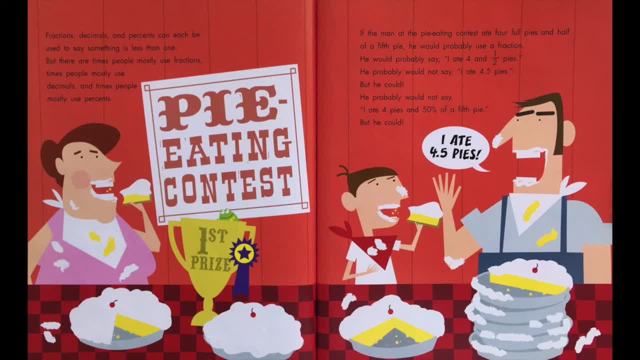 Fractions, decimals and percents can each be used to say the same thing. You can also change the denominator. You can also change the denominator. We can also change the denominator. Now you can change the denominator, For example. make some capital this way. 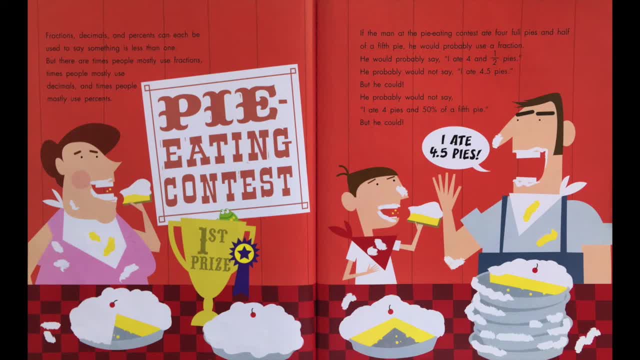 Let's say you want to say something less than 1.. So say something less than 1.. But there are times people mostly use fractions, times people mostly use decimals and times people mostly use percent. If a man at the pie eating contest ate 4 full pies and half of a fifth pie, he would probably 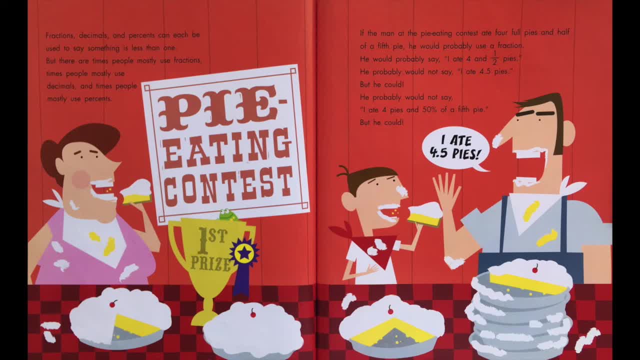 use a fraction, He would probably say I ate 4 and 1 half pies. He probably would not say I ate 4.5 pies, but he could. He probably would not say I ate 4 pies and 50 percent of a fifth. 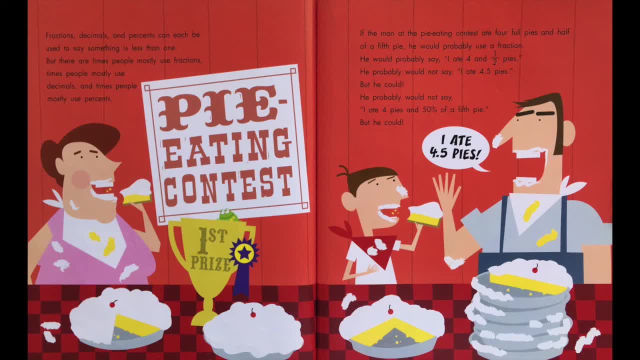 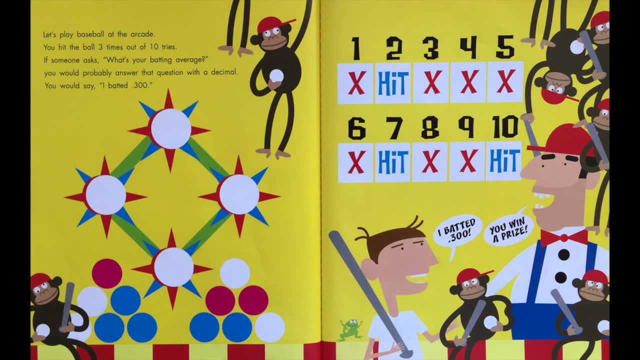 So we make the�� into a fraction. fifth pie, but he could. Let's play baseball at the arcade. You hit the ball three times out of 10 tries. If someone asks what's your batting average, You would probably answer that question. 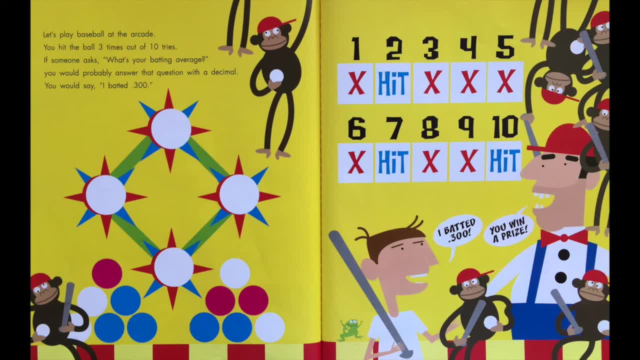 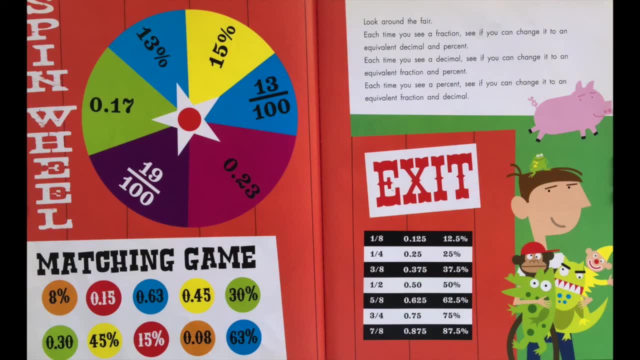 with a decimal, You would say I batted 0.300.. Look around the fair. Each time you see a fraction, see if you can change it to an equivalent decimal and percent. Each time you see a decimal, see if you can change it to an equivalent fraction and percent. Each time you see a.